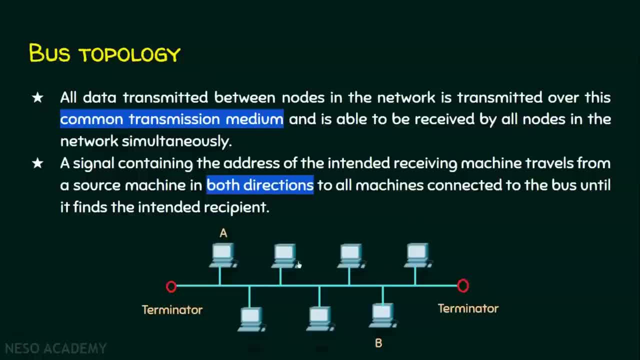 Now, the problem with this approach is: if A wants to send some data to B, everyone will receive a copy of the data signal, including B, but all others will deny or reject this packet. Why? Because this data signal is intended to the recipient B. 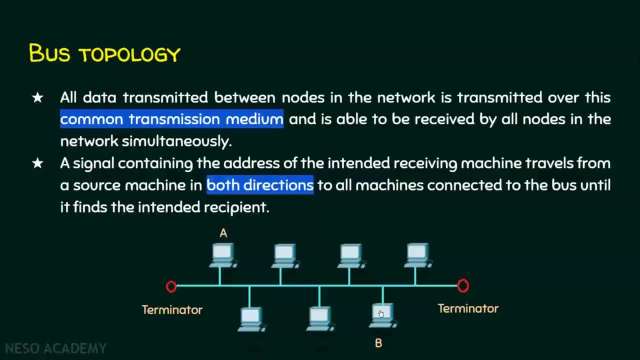 and not to anyone else in the network. So now we will see what is a bus topology. as per the definition, All data transmitted between nodes in the network is transmitted over this common transmission medium. This is the common transmission medium, and all nodes will receive this signal simultaneously. 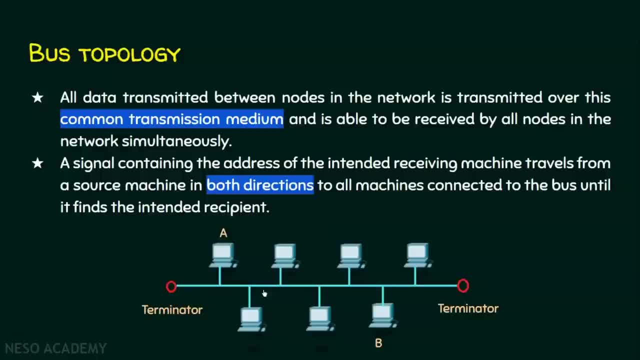 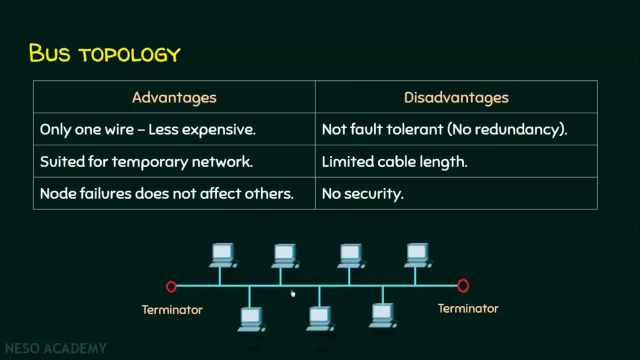 This transmission medium is capable of sending as well as receiving the data, So the data flow in this transmission medium is bidirectional. It means data can flow in both directions. We will see the advantages and disadvantages of bus topology, Since there is only one wire or the cable involved in this transmission. 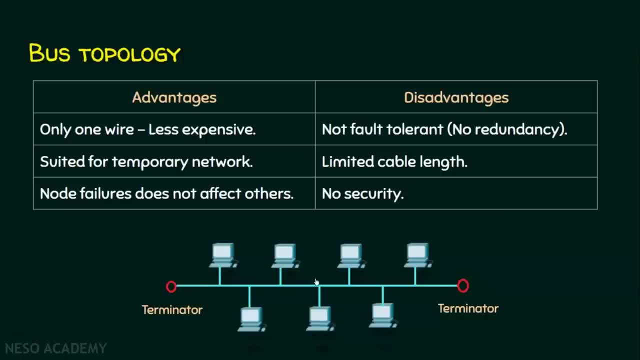 it is less expensive. At the same time, if you are going to construct a temporary network where this is not going to last for a long, then you can go for bus topology. Another advantage of having this network is that if any node failure- please watch this- this is a node failure. 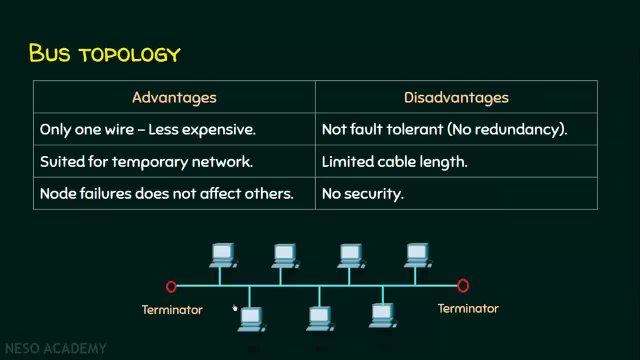 and this node, failure does not affect others. And these are all the advantages of bus topology. There are some disadvantages with this network And this is obviously not a fault tolerant network. We have already seen what is a fault tolerant network. Fault tolerance means if there is a failure. 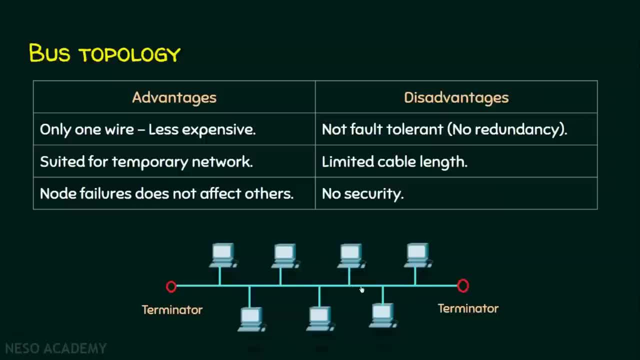 and this failure should not affect others. But if this link, this transmission medium is failed, obviously the entire network goes down At the same time, if this node wants to send some data to this node and there is a problem in this line. 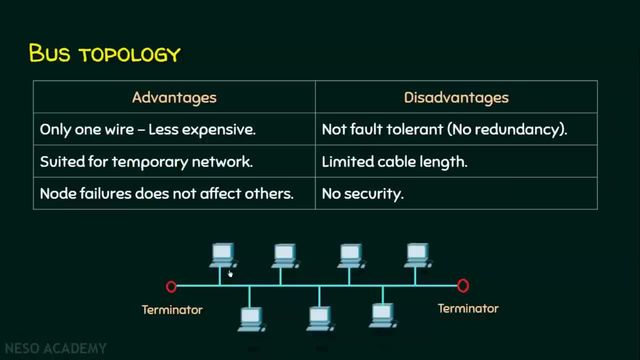 So communication here can take place, but the communication between this place will not happen. Why? Because this is not dealing with any alternative technique. Why? Because this is not dealing with any alternative technique. Why? Because this is not dealing with any alternative technique. 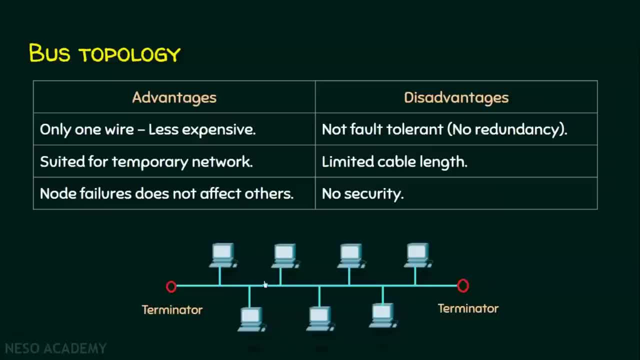 The only way for this computer to reach this computer is this line And there is no redundant line, And that is why this network is not a fault tolerant network. At the same time, the cable length is limited to certain range. Also, I have already mentioned 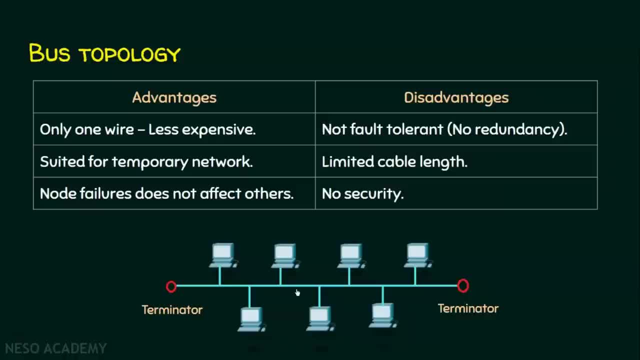 if this node wants to send some data to this node, everyone participating in this network will receive a copy of this signal. So there is no security in this approach. And that's the advantages and disadvantages of bus topology. And coming to the second topology, the ring topology. 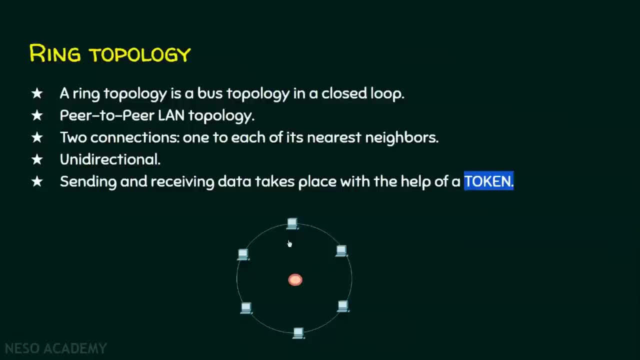 a ring topology is a bus topology, but in a closed loop. If you observe, this is a bus topology, but this is a closed loop. So here the nodes involved are peer-to-peer LAN topology nodes. It means there is no one superior in this network. 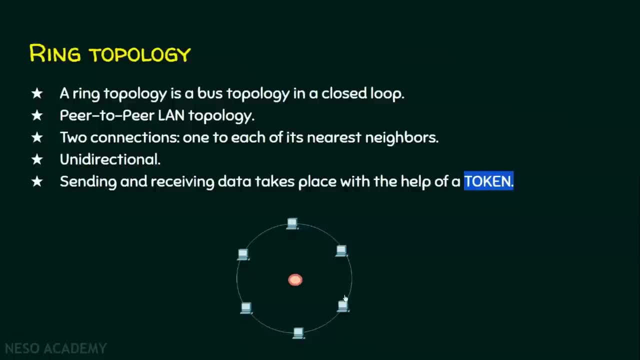 and there is no one inferior in this network. All nodes are with equal rights And that is why we call these nodes are peer-to-peer nodes, And every node will have two connections, One to each of its nearest neighbors, And the communication is always unidirectional. 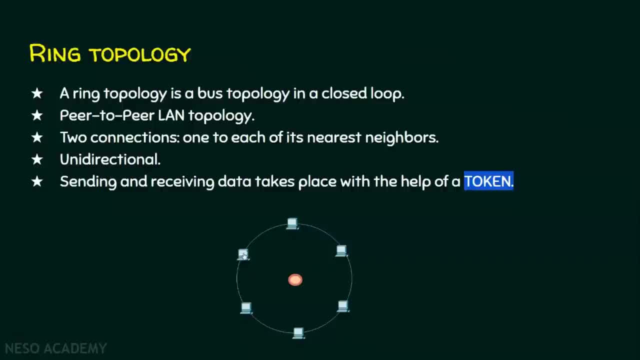 Suppose, if this node wants to send some data to this node and the network is set up like the flow of data should be in this direction, and this node will send this data to this node and this node will forward the data to this node. 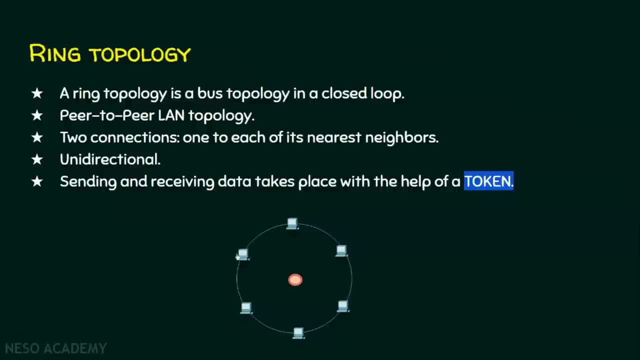 this node, this node and finally it will be received by this node. The communication will not happen directly like this. The communication will be like this because the communication pattern of ring topology is always unidirectional, And you may ask me how this communication will happen. 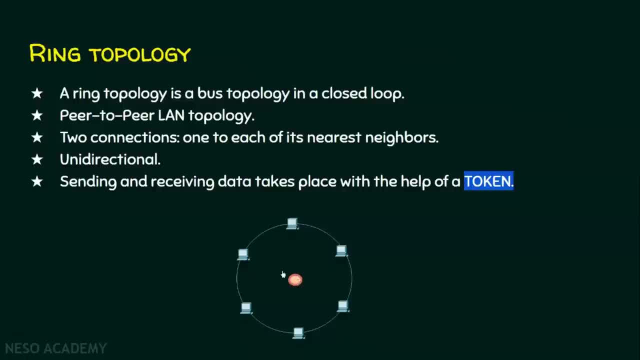 It is with the help of a token. That is why we call this topology as a token ring topology. Now we will see how sending and receiving happens with the help of this token. Let this be a token. Whoever has this token, it means it's their turn to send data. 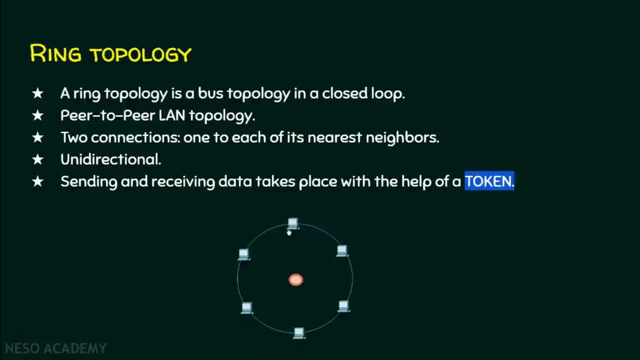 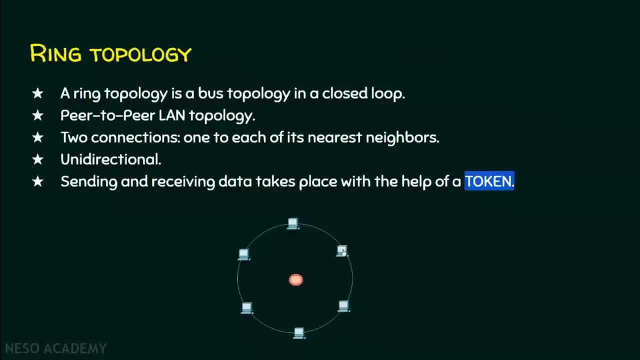 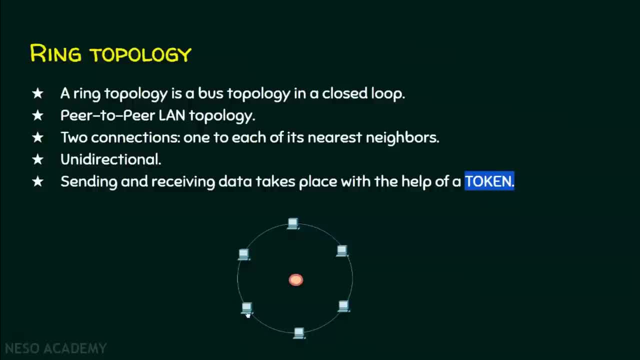 And this token will be circulated throughout this network. It means whoever holds this token, it's their time to send their data And this is how all nodes gets opportunity to send or receive the data. Just watch this example: The token is circulated throughout this network. 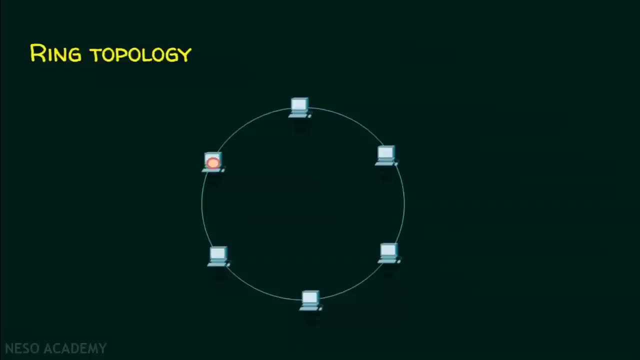 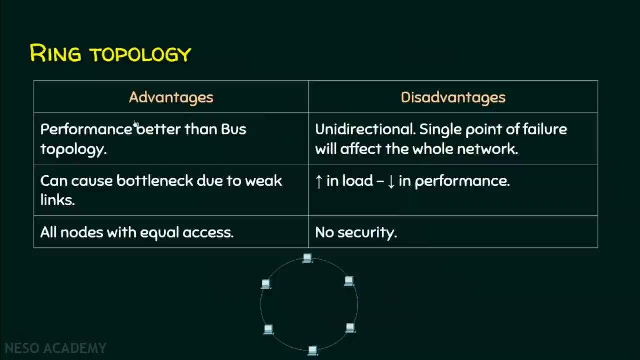 It means whoever is holding this token, it's their turn to send the data. And this is what exactly a ring topology is. Coming to the advantages of ring topology: it has better performance than bus topology because it is in a closed loop. 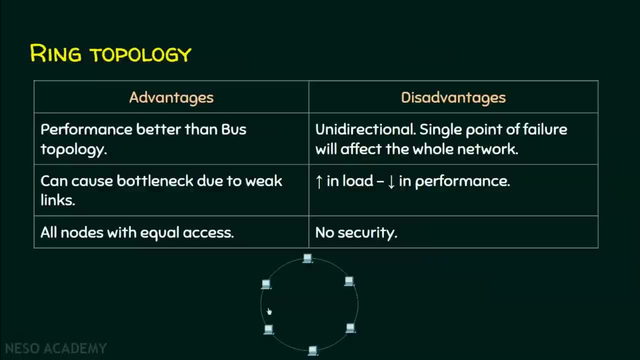 But the problem is, if this link is a weak link, this ring topology causes some bottleneck in the network because of this weak link. At the same time, all nodes are having equal access, which is considered to be one of the advantages of ring topology. 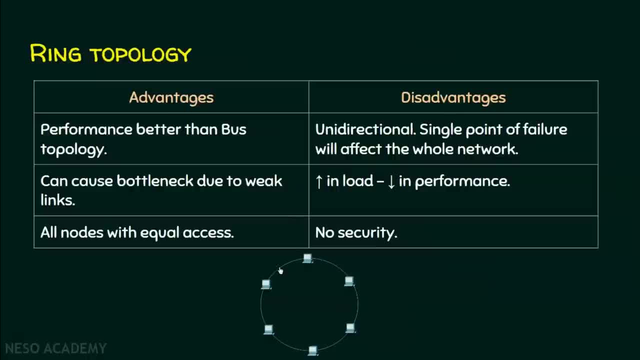 And coming to the disadvantages of ring topology, I have already mentioned. it is unidirectional, Say. if this node wants to send some data to this node, it is very easy to send this way. But ring topology is a unidirectional communication pattern. 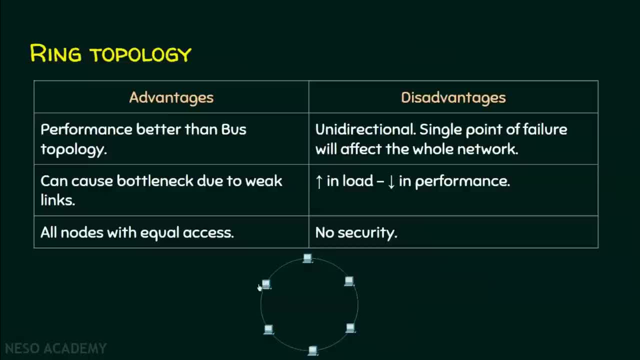 It has to send the data by crossing these many nodes and finally reach the destination, And one of the disadvantages is being unidirectional At the same time. a single point of failure say this link is failed, So the entire network is disrupted because of this. 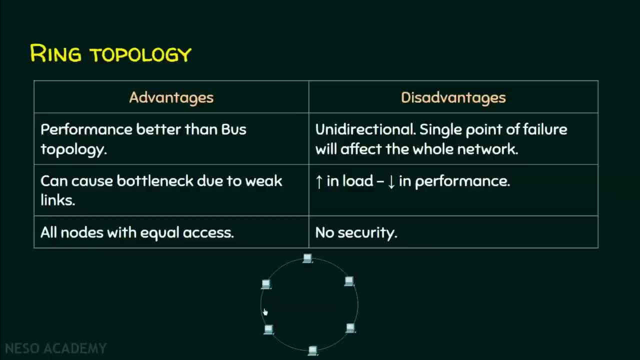 A node failure or a link failure will definitely affect the entire network And this is what the primary disadvantage of a ring topology: If there is very high load in the network, then the performance of the network is getting degraded. If this is going to send some confidential data, 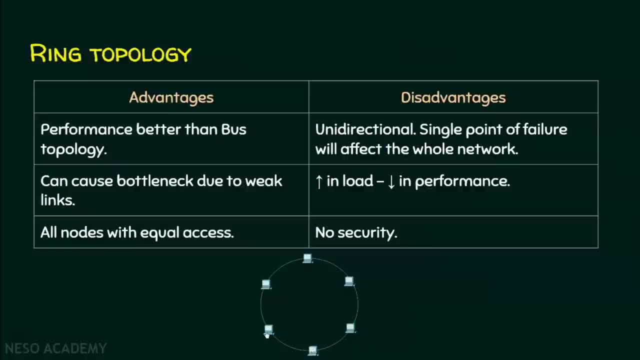 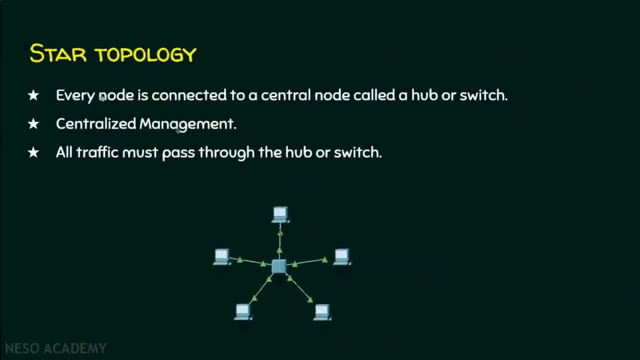 to this computer, but again this has to cross so many intermediary nodes in order to reach the destination And obviously there is no security in this ring topology. Now we will see the third topology, the star topology. In this case, every node is connected to each other. 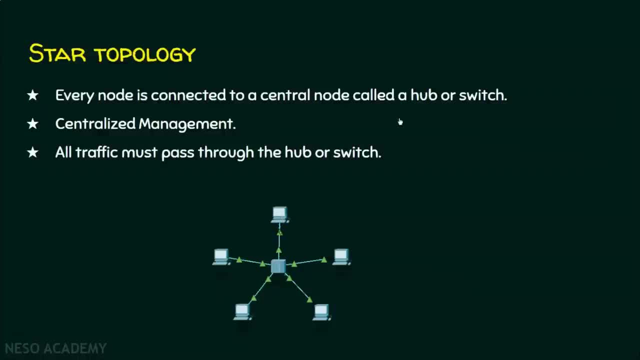 but not directly, but with the help of a central node. This central node can be a hub or a switch. We will deal elaborately about hub and switch in the upcoming lectures. For tyme being, you just make a node of this hub. 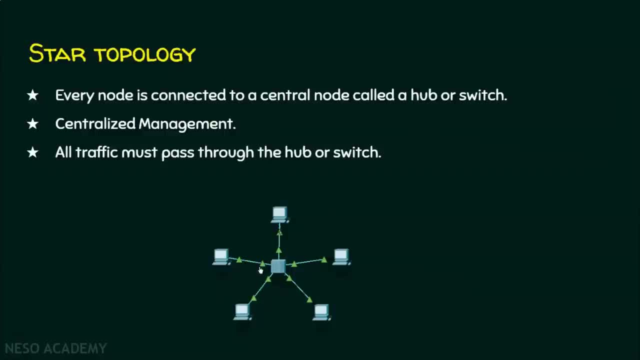 or a switch as a central device or a central node and this is going to do the anti-centralized administration And all traffic must pass through the hub or a switch, Suppose if this node wants to send some data to this node. so obviously this is going to send the data to the central node. 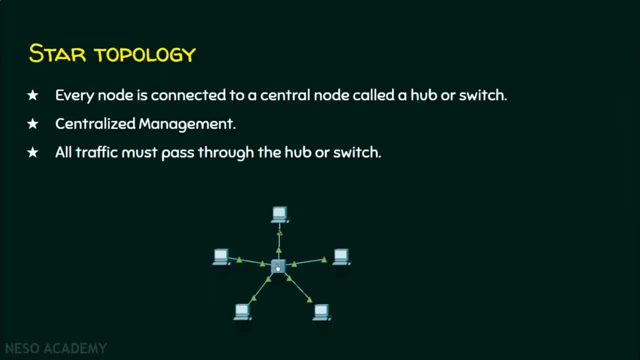 which is the hub or the switch here, and it is the responsibility of this node. So obviously this is going to send the data to this central node, which is the hub or the switch here of this hub or switch, to forward the data to this node. that is the destination. 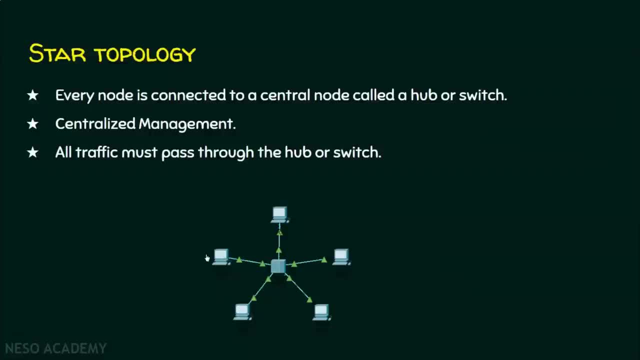 If you observe keenly, in the previous cases there were chances for other nodes to receive a copy of the data, But here, if this node wants to send some data to this node, and this is going to be the path of this communication and there is no way for others to hear this communication or see this communication. 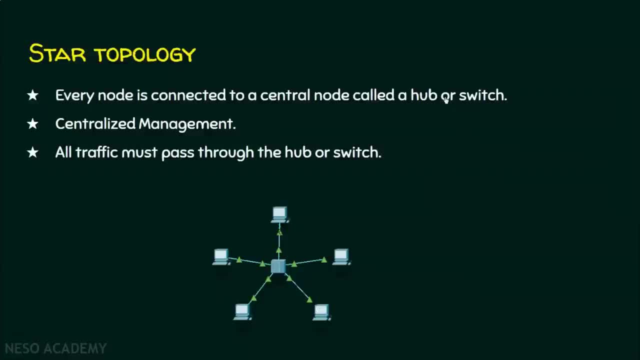 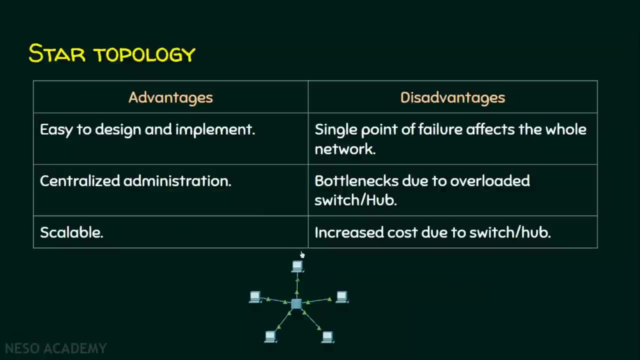 But there are some differences between hub and switch which will be dealt elaborately in the next lecture. Coming to the advantages and disadvantages of star topology, it is definitely very easy to design and implement. At the same time, we have a centralized administrator here. 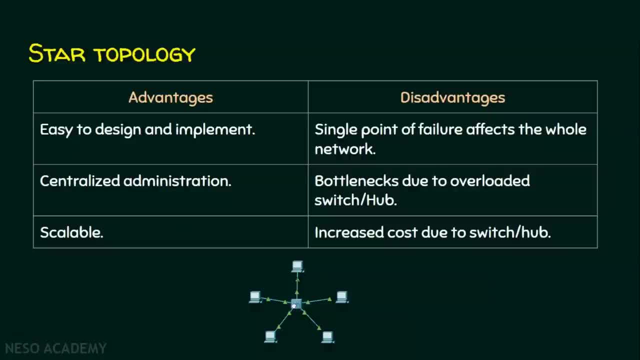 This is the hub or a switch. If this switch has 24 ports, for example, you can connect 24 computers to this switch. If you find that 24 computers are not sufficient, you have 50 more computers, you bring another switch and connect all the computers to that switch. 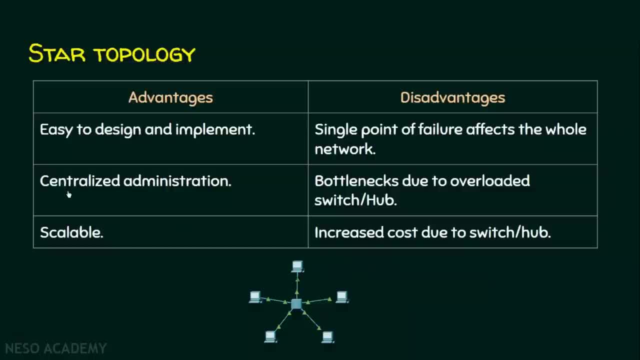 and again make a communication between this switch and this switch So that this network becomes a scalable network. So star topology is easy to design and implement and there is a centralized administration and it is a scalable network. And star topology has a serious disadvantages too. 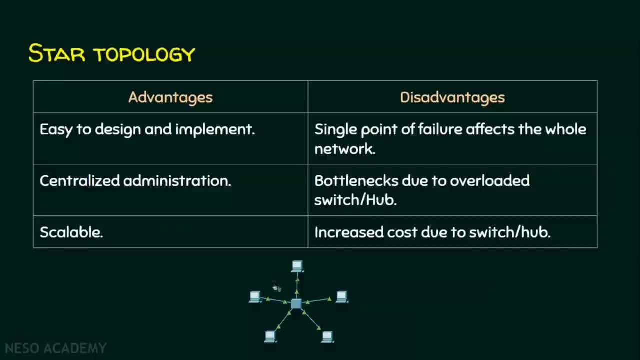 A failure in this central node will affect the entire network. If this node, that is, the switch or the hub, is failed, no communication can take place At the same time. if this node is overloaded, with lot of traffic and lot of processing. if this node is overloaded, with lot of traffic and lot of processing. 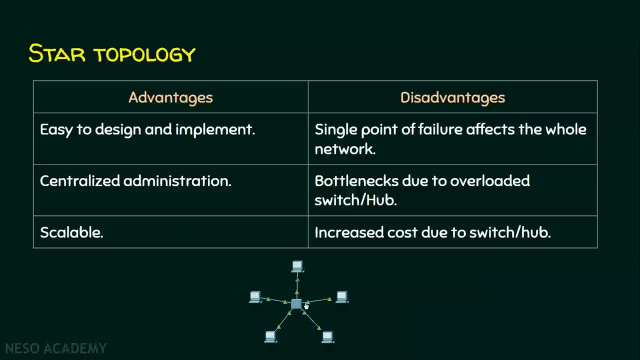 If this node is overloaded with lot of traffic and lot of processing, then the communication or the performance is affected. That is what we call as a bottleneck. You have to spend some money for purchasing this hub or a switch, So obviously it is going to increase the cost. 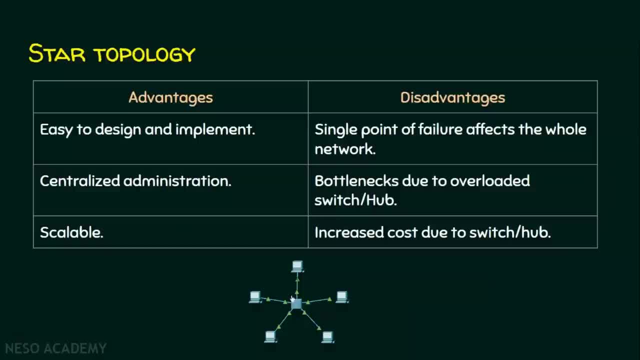 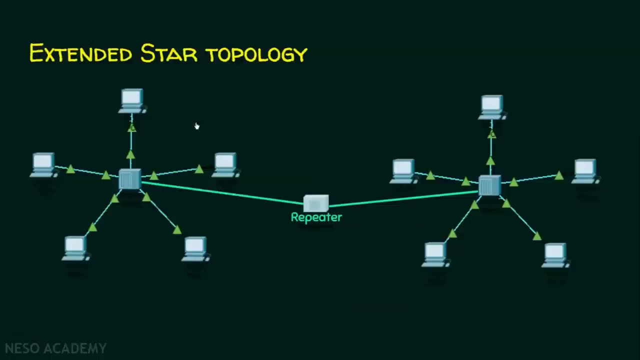 So there are some disadvantages. A single point failure is going to affect the whole network and there can be bottlenecks due to a overloaded hub or switch. At the same time, you have to spend more for purchasing this hub or a switch. We can also have a variation of a star topology. 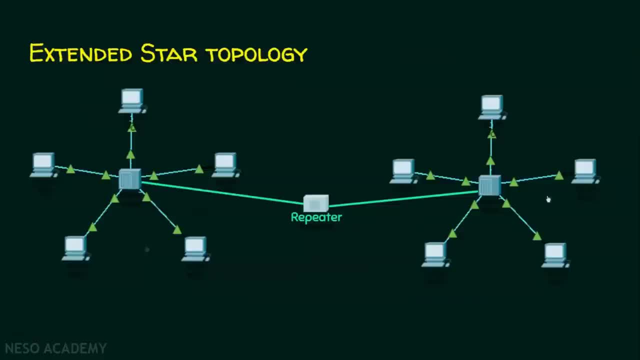 Like this: this is one star topology, another star topology. You can connect these two star topologies with the help of a repeater. We will see about repeaters in the next lecture. Now the point to note is that two or more star topologies 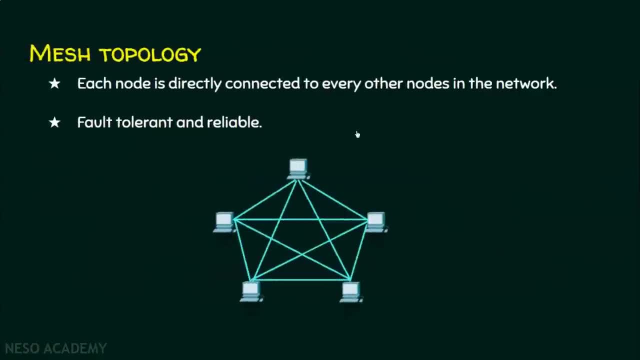 can be connected with each other like this. And the last topology of the session is the mesh topology. If you observe, there are five nodes And if you observe this node is having a link to all other nodes. Likewise, this node is having a link to all other nodes. 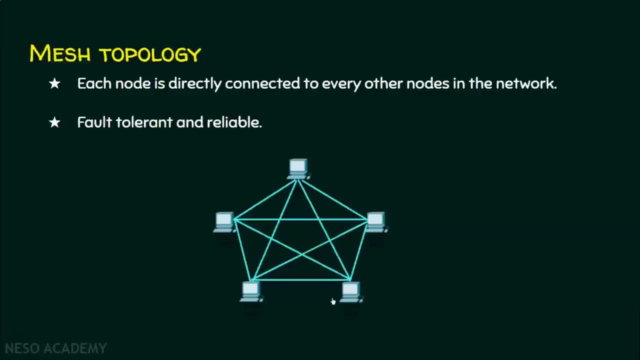 Likewise, this node is having a link to all other nodes. So, if you observe keenly, this is the topology where each node is directly connected to every other nodes in the network And thereby it provides 100% fault tolerant and reliability. 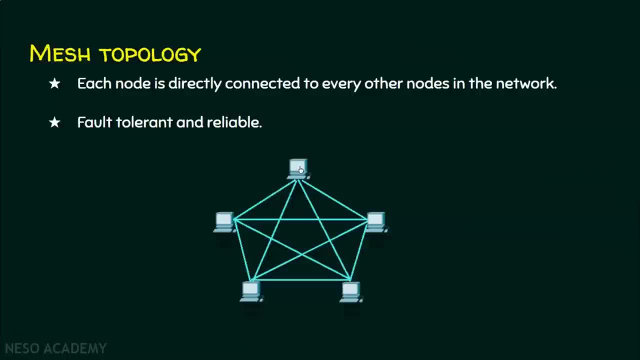 Suppose, if there is a link failure encountered here and this computer has another way to reach the destination If this link is failed. this computer has so many ways to reach the destination. This is one way, This is another way And this is another way. 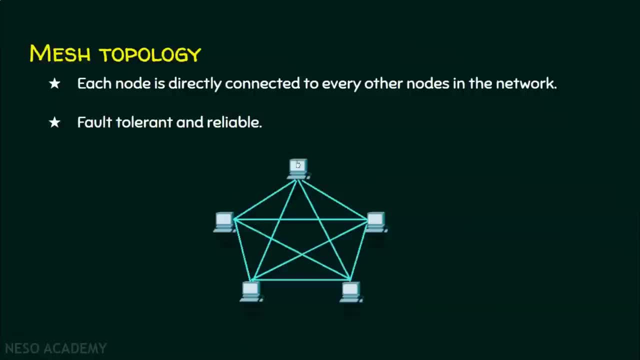 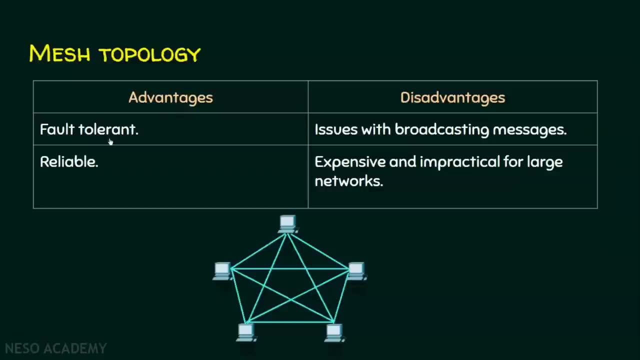 And this is another way. There are so many ways for a node to reach the destination. We will see the advantages and disadvantages now. The advantages of mesh topology are: it is fault tolerant. It means a failure is not going to affect the network. 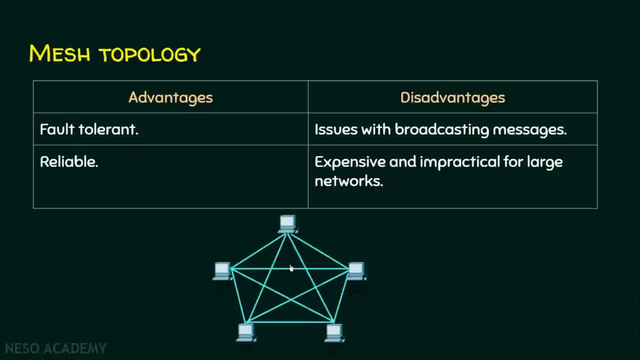 At the same time, you can rely upon this network because somehow your data will definitely reach the destination, even if there are link failures And coming to the disadvantages if this is going to send a broadcast message. broadcasting means one sender, all receivers. 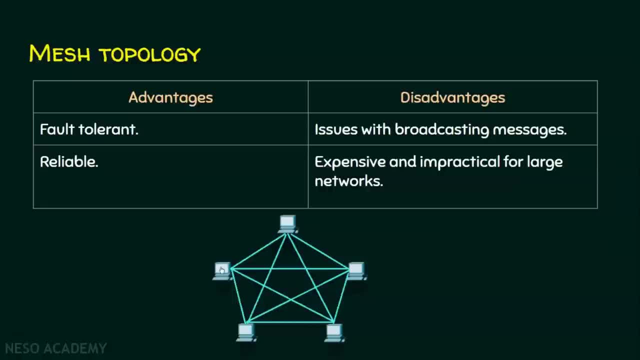 This broadcast will be forwarded to everyone in the network. Again, this guy is going to do a broadcast to everyone in the network, The same broadcast which is sent by this computer, and it will also be received by other computers, and those computers are going to forward the same broadcast to the sender. 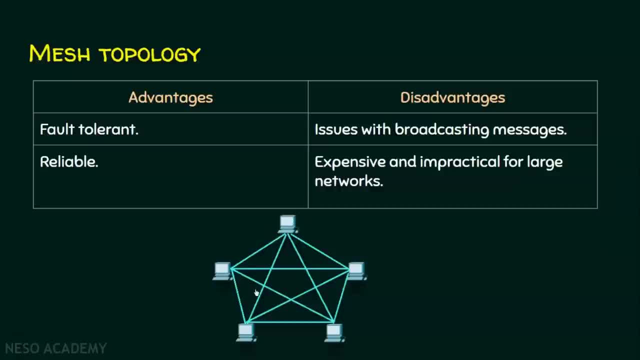 There are some issues with the broadcasting, Since mesh topology involves a lot of links, so it is obviously an expensive one. At the same time, for smaller networks, this mesh topology is not going to be able to send a message to the sender. 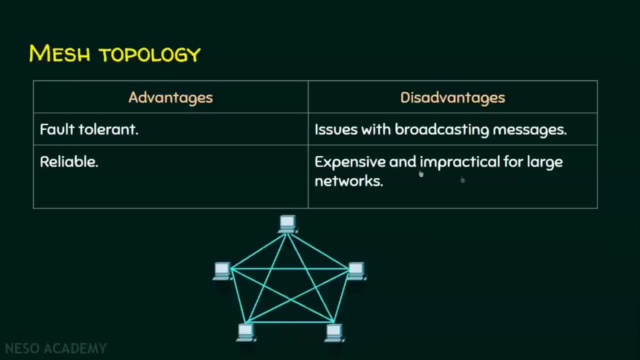 It is going to be forwarded to the sender. So this mesh topology will work fine And it is really impractical if your network involves 1000 or 2000 computers or more than that. These are all the disadvantages of a mesh topology.